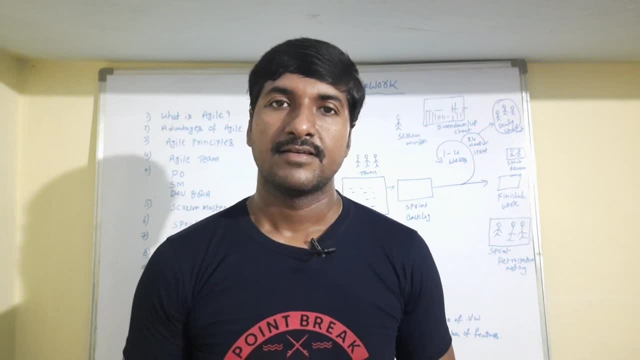 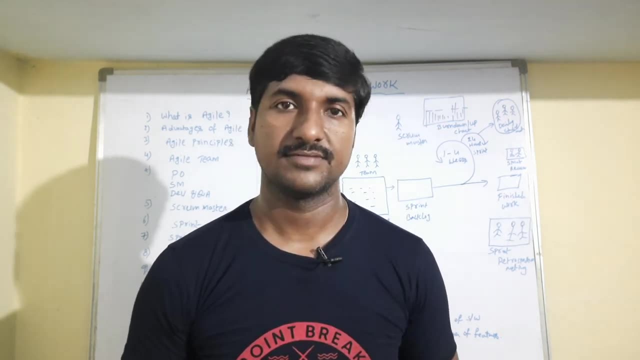 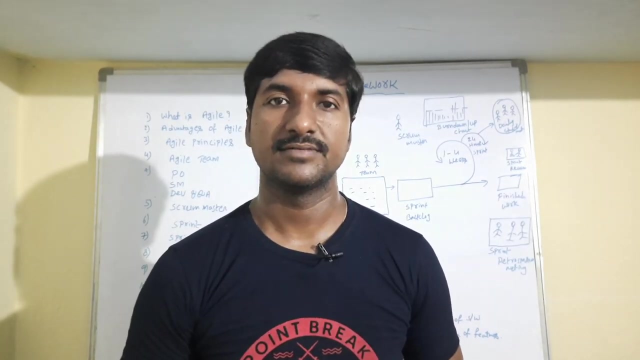 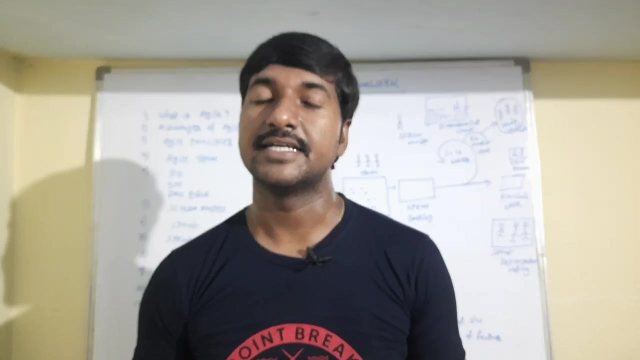 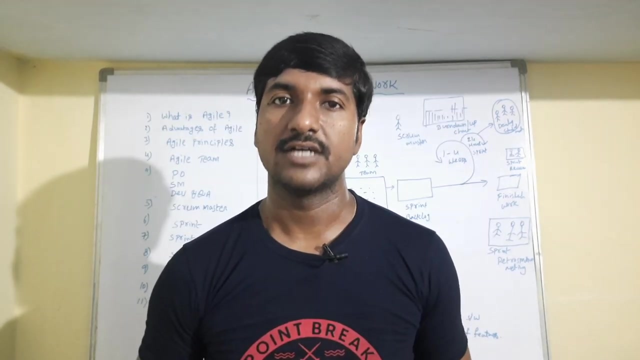 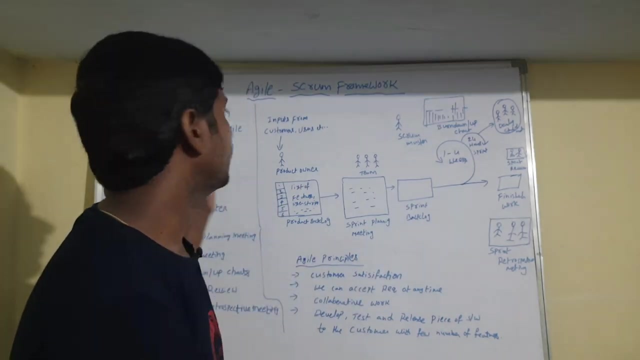 are there in SDLC. the same thing, the same process, will repeat it. that is nothing but iterative in agile process. okay then what about incremental? incremental means we're adding the new features. that is the incremental. and ics sayımız nu Docker, don't share anything. triple multiple: 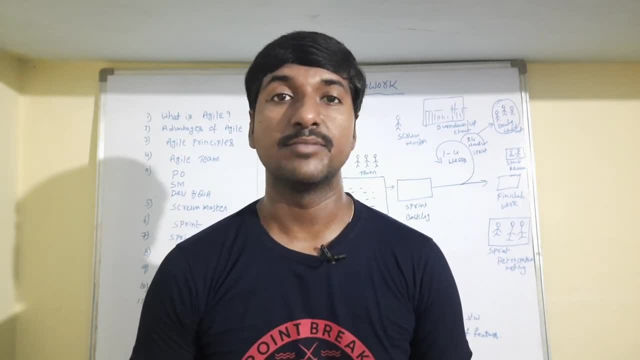 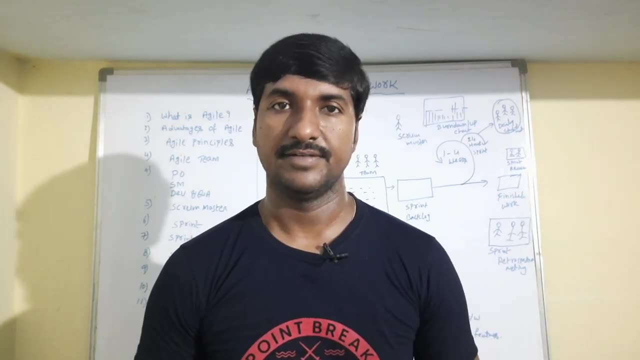 anything to do with each one. okay, so technically speaking as well is nothing, but it is a innovative and incremental process. guys to develop the projects are to implement the projects in a IT companies. okay then, what some? uh, there are some project methodologies are there, but nowadays everyone is recommended. 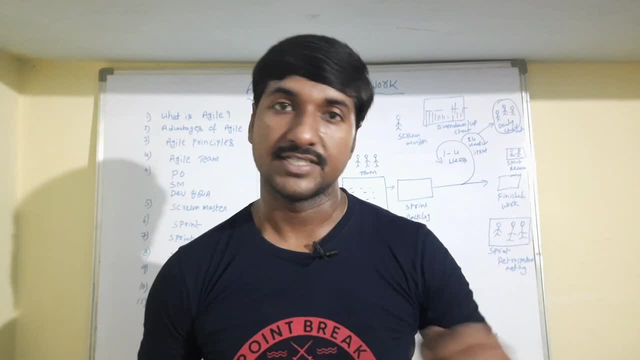 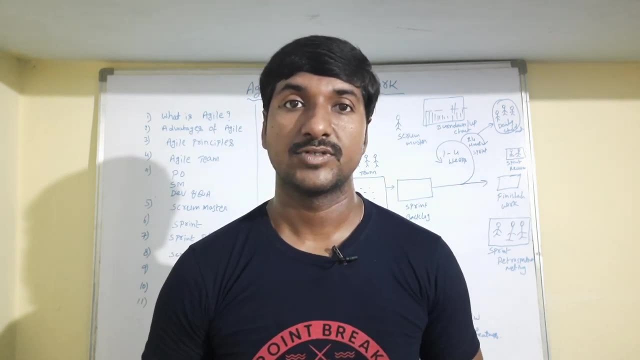 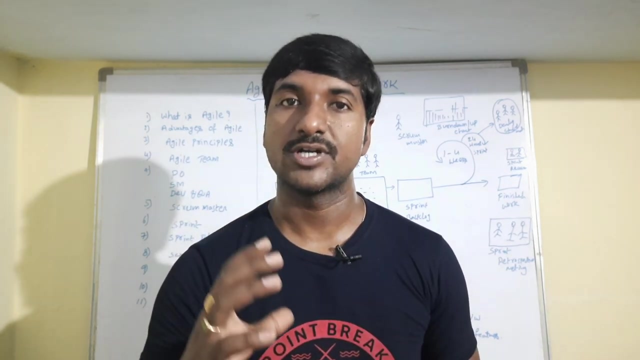 to use agile only because of these advantages, guys. the first advantage is the customer: no need to wait for long time, guys, to get the product or software. okay, so he can get his product or software for every two weeks or three weeks. and the second advantage is you. 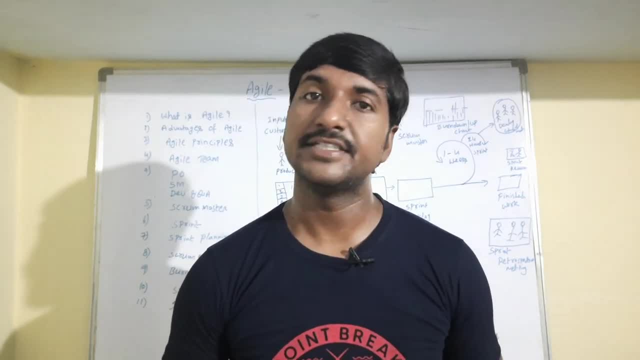 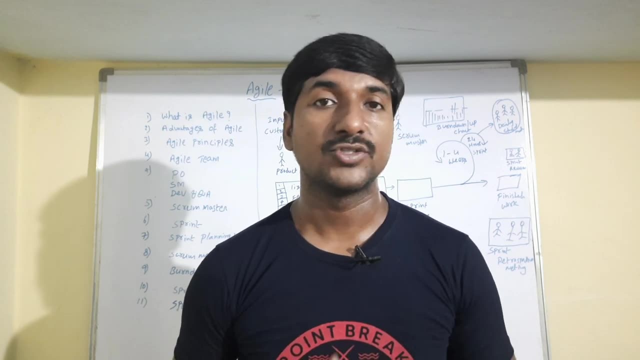 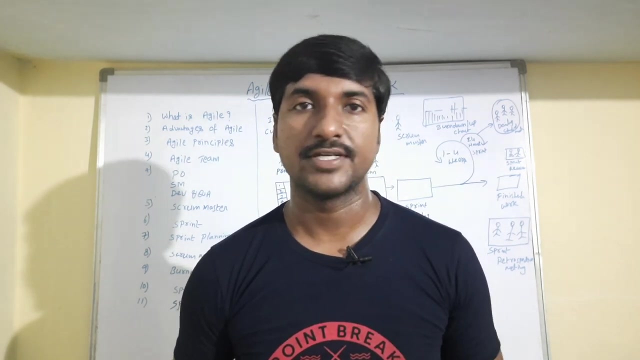 can change your requirement at any time, place, any stage. but in earlier, traditional project methodologies there is no chance, are there, there is no opportunity to change your requirement in the middle of the project. but in agile project methodology you can change requirement or accommodate the requirement at any stage of the project. 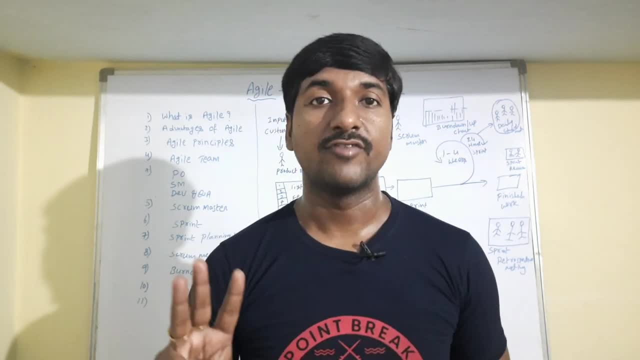 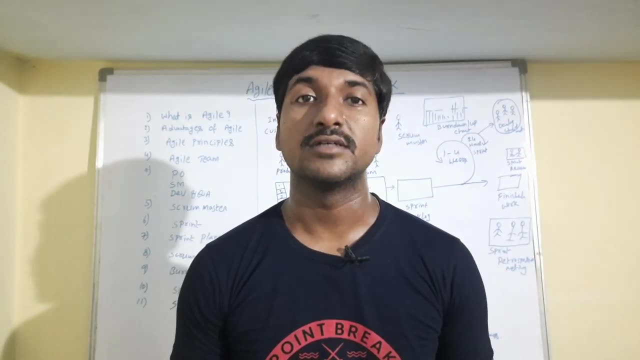 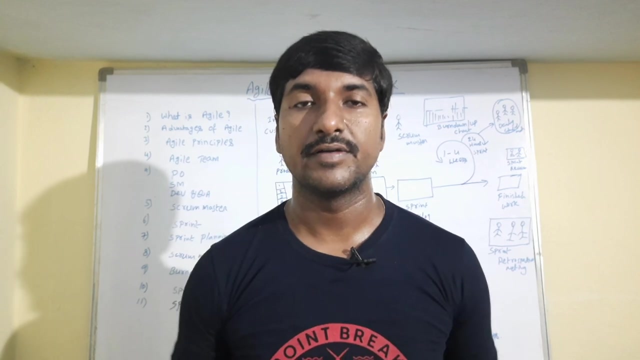 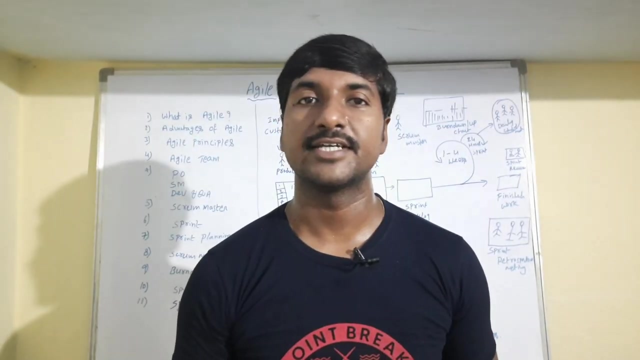 no problem at all. and the third advantage is it's a collaboration work guys. collaboration work means communication between product owner development team and qa team and some other admin teams. it works, everything happens in the communication. you can easily communicate with your team members. that is nothing but a collaboration work, guys. okay, that is also. 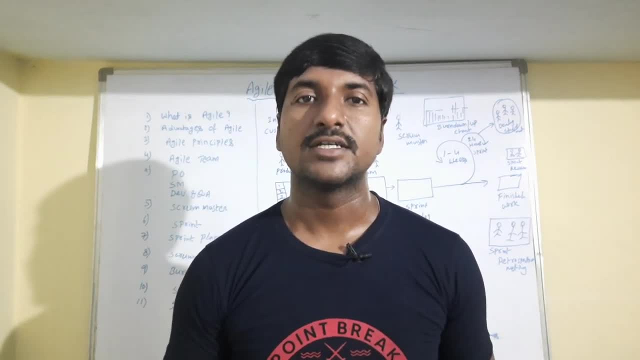 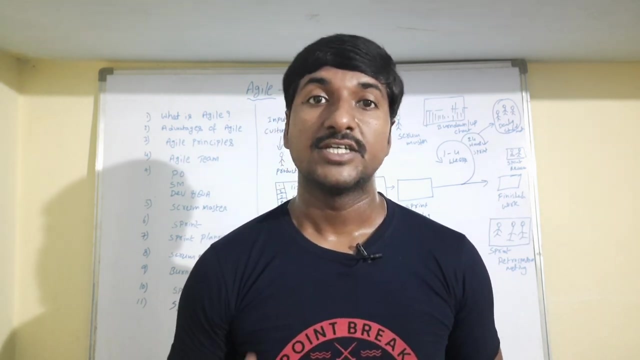 main advantage of agile process. so your product owners, scrum master and qa team and dev team, and also some admin people- all are working together to complete the project. that is the main advantage of agile process. and one more advantage is you can expect the piece of software for every two weeks or three. 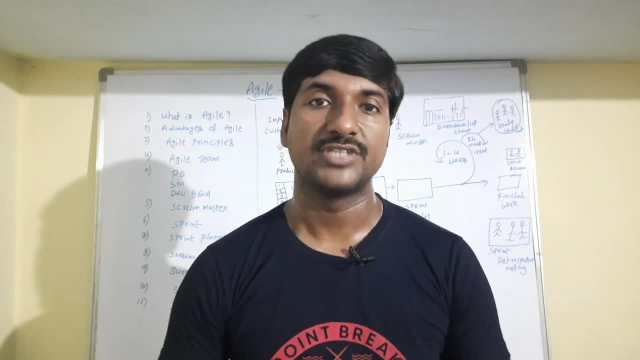 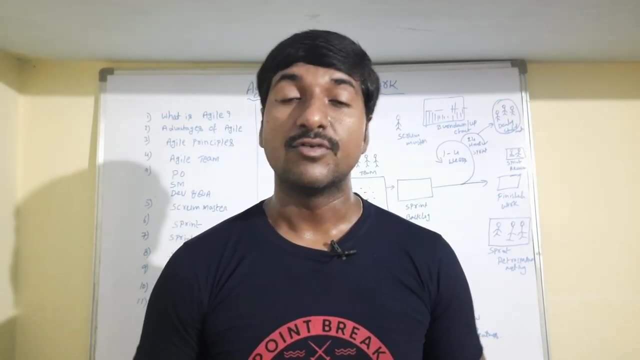 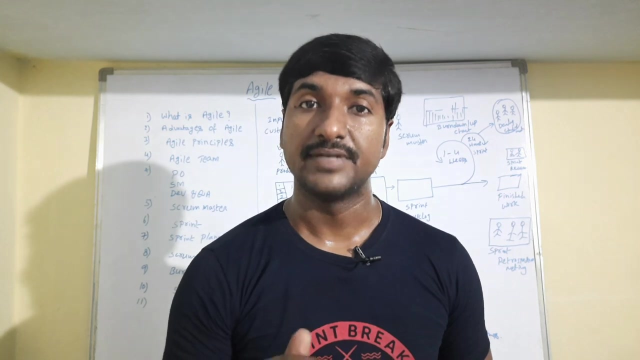 weeks guys. so therefore, customer having a good satisfaction with agile process. so these are the four main advantages of agile guys. next one is we will see some agile principles guys. so based on these agile principles only every it company follows, based on these principles, guys, to develop their projects. okay, so i will. 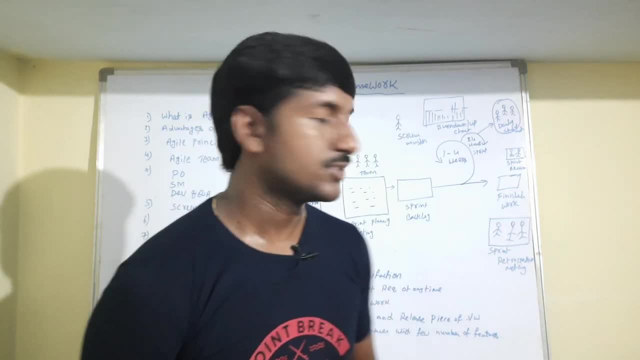 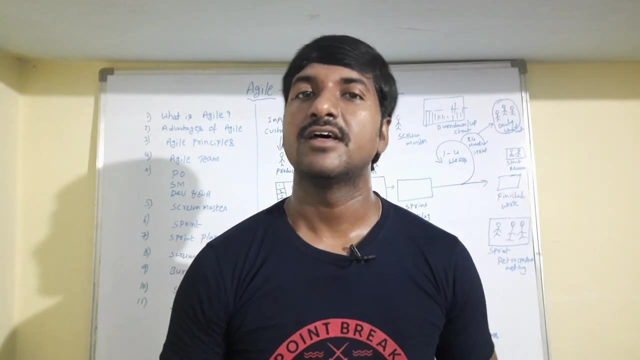 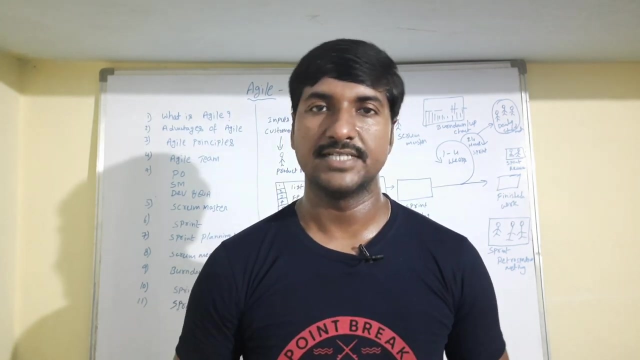 tell you a very important agile principles. the first one is customer satisfaction. that means customer no need to wait for long time to get the product. that is the main principle. that is the main agile principle, guys. customer no need to wait for a long time, he will get immediately, he will get. 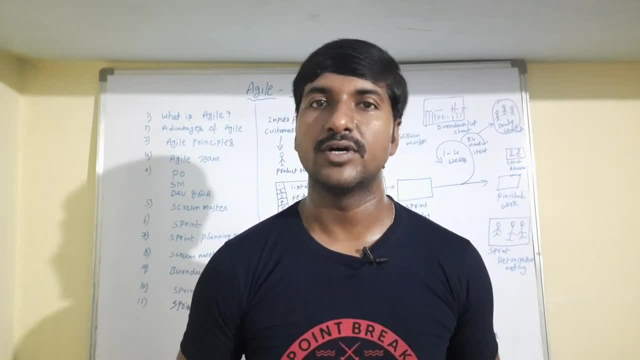 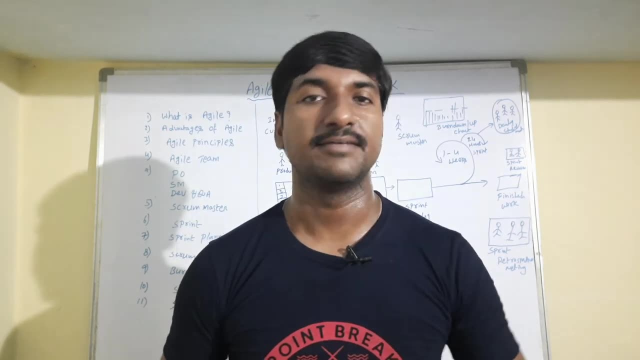 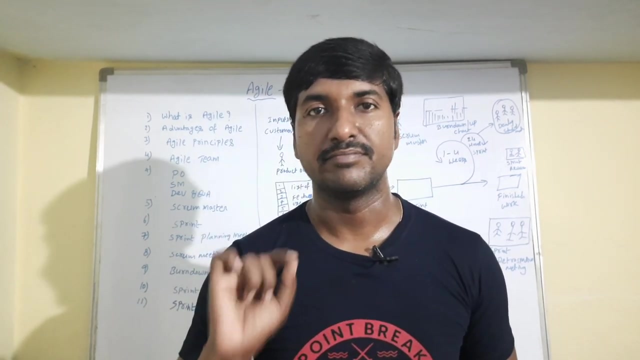 his software product immediately for every two or three weeks, okay. and the second principle is: we can accept the requirement at any time. that means we can change the requirement at any stage of the time. that is also one of the main agile principle. and the third one is: 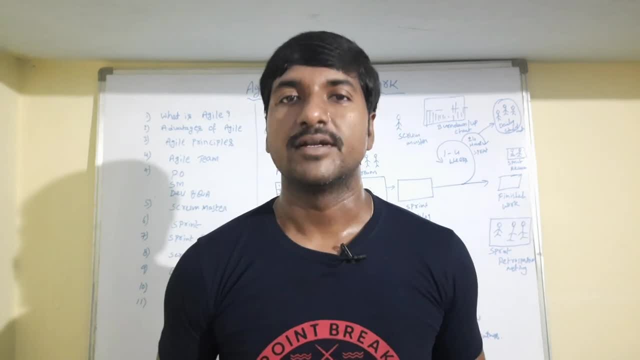 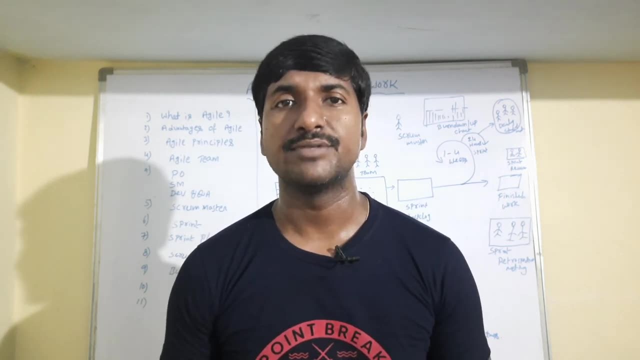 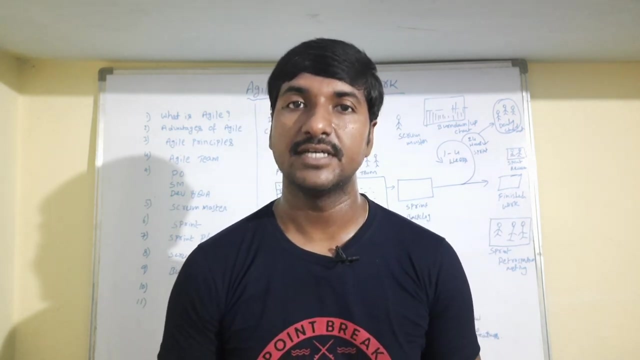 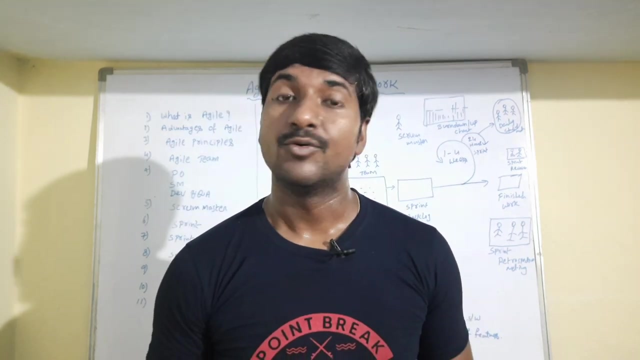 collaborative work. that means everyone- product owner, scrum master and some business people and also dev team, qa team. all are work together. that means communication happens very easily between the team. okay, and the next one is the next main principle is we can develop, test and release the piece of software to the customer with feweráfication and out of abuse. it only allow it is the搶 deal, the dealership, and on that, 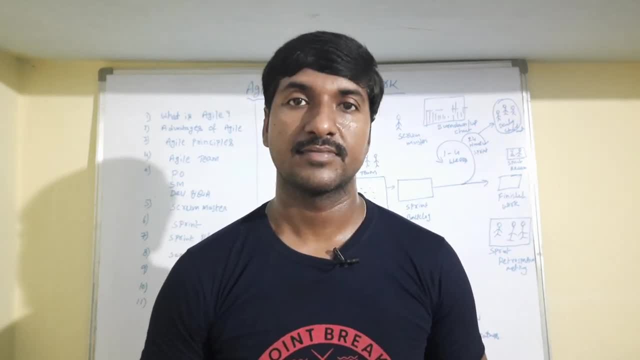 means we can hurt because on the logins: okay, all thebearable friends to go to okie a. you guys for test, andadow it off. well, i will see you in one of the next with a few number of features. guys, for every 3 weeks or 4 weeks, customer, get some piece. 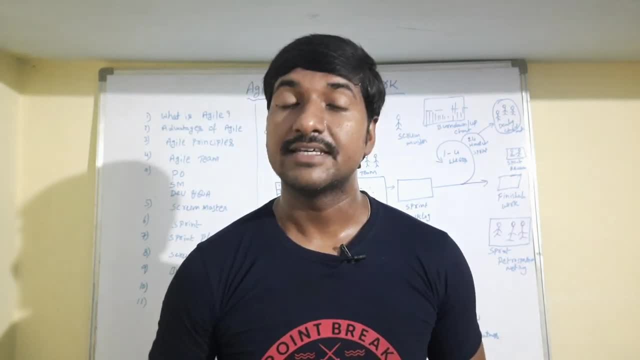 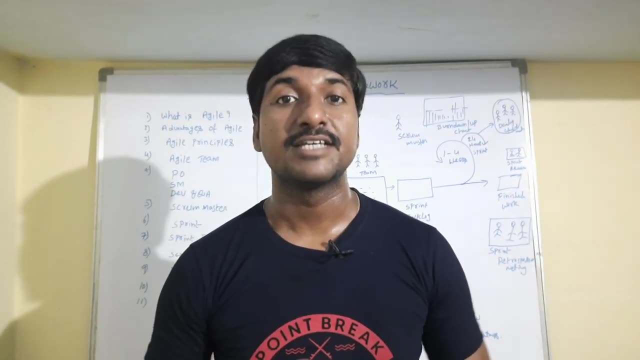 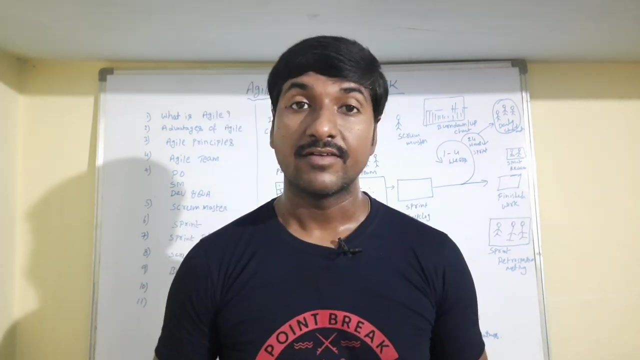 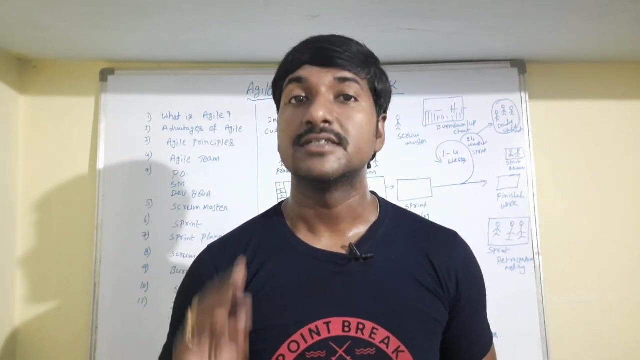 of software. okay, so these are the main agile principles, guys. okay, then what is the scrum? so scrum is nothing but a framework to build a software product by following agile process. then what is the scrum team? the scrum team includes 5 to 10 members, guys. product owner. 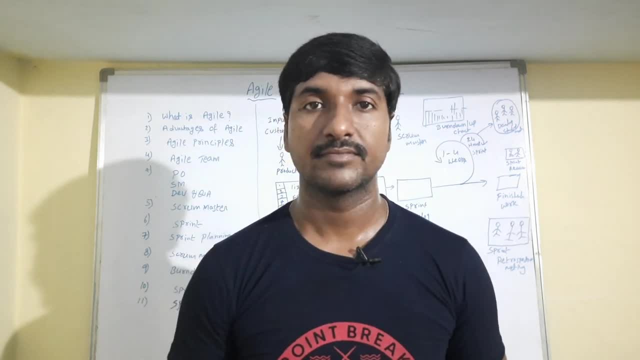 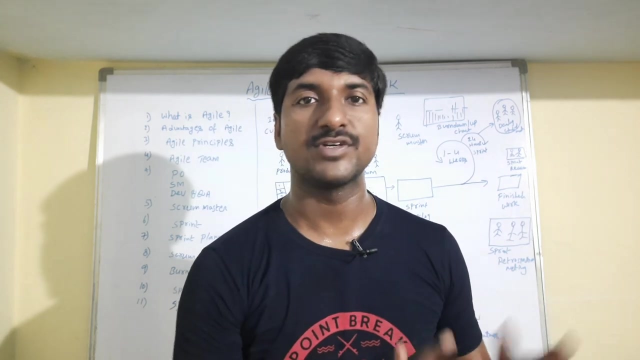 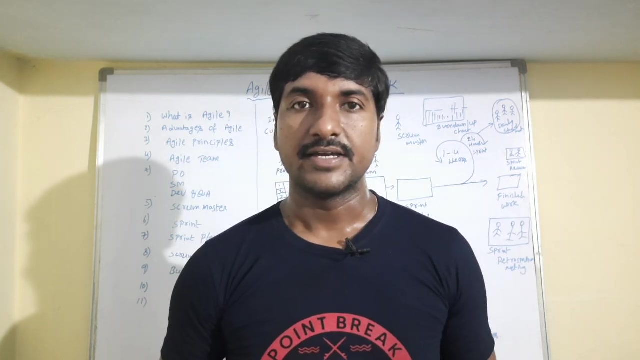 scrum master dev team and qa team. okay, so then what is the main responsibility of product owner? so the product owner is a special designation in iit companies. guys, he has some specific role. is there? he has some specific designation in iit companies. okay, so he is. his main responsibilities are he is to communicate with the end users stake. 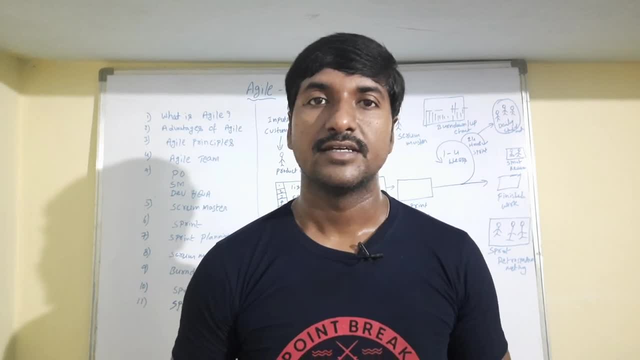 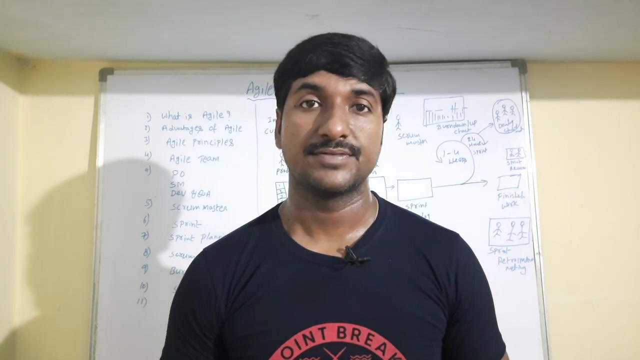 holders: okay, or clients: okay. he will collect the data. he will collect the user requirements: okay, he will define the features. so the main responsibility of product owner: he defines the product features and he is also responsibilities to prioritize the listing of product features, okay, and this what we are helping with: biggest behalf for product owner andmm everything, because 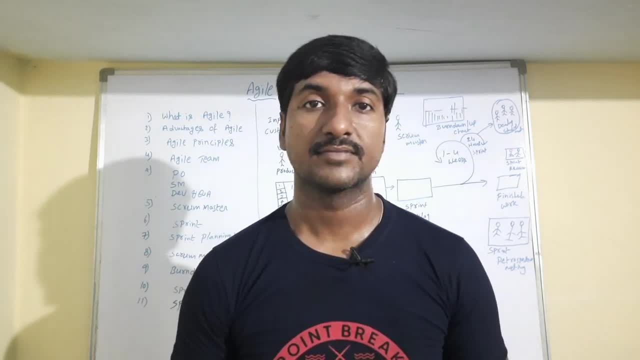 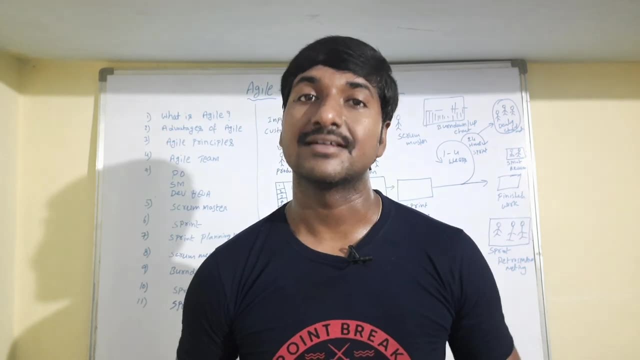 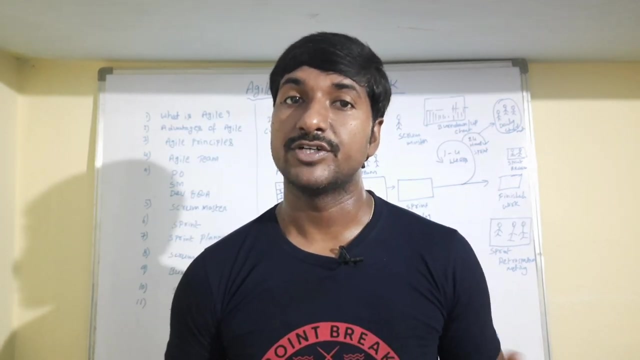 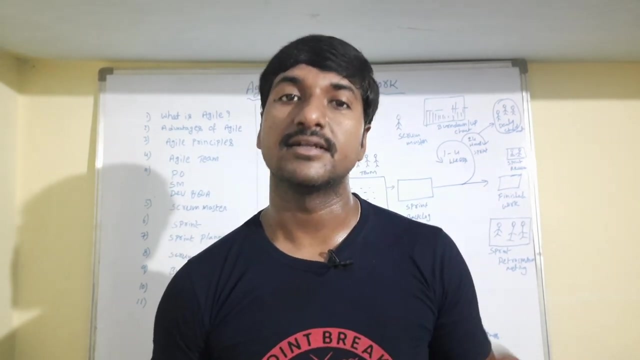 of features or user stories. okay. and also he has a one more responsibility: he can accept or reject the the status of the product in case the product owner he is not satisfied, whatever we develop the product, he may reject the product also. he is also authorized person who can accept or reject the. 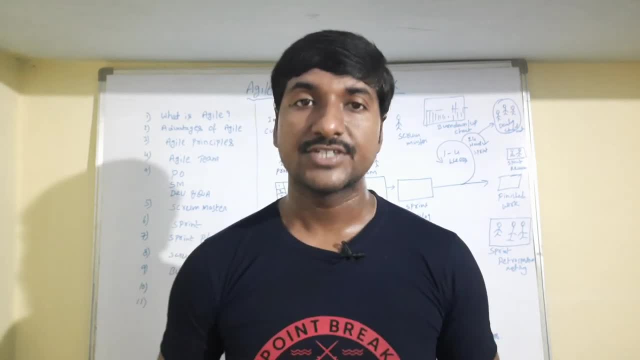 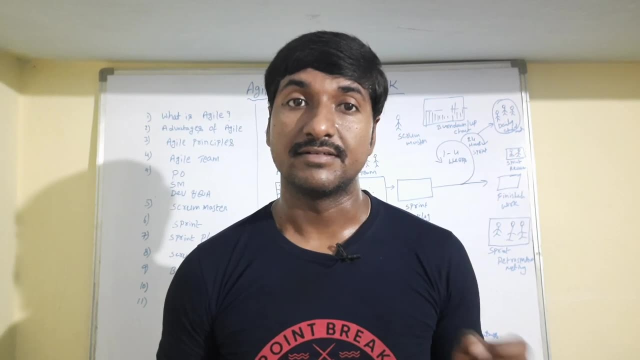 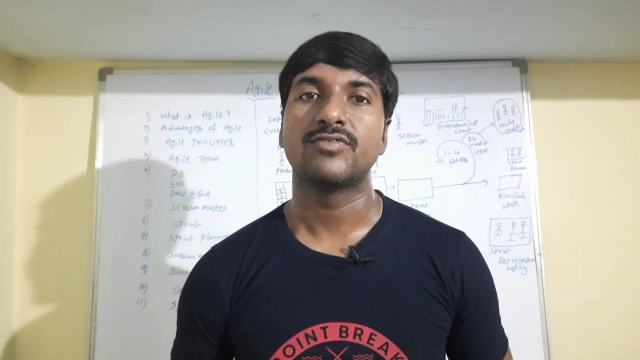 product. okay. and the next one is scrum master. who is a scrum master? scrum master is nothing but so scrum master. he is drive the as a principles. he is facilitating and drive the agile principles. he will take care of all entire project, whether the project is. 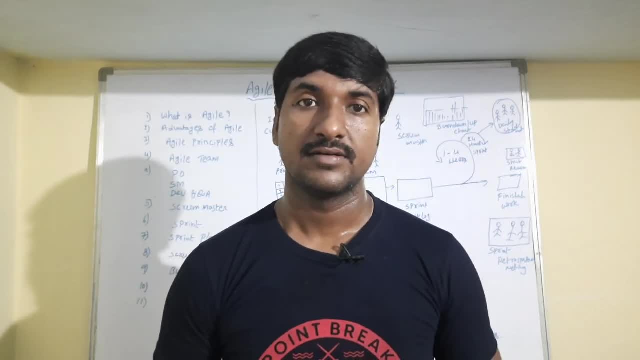 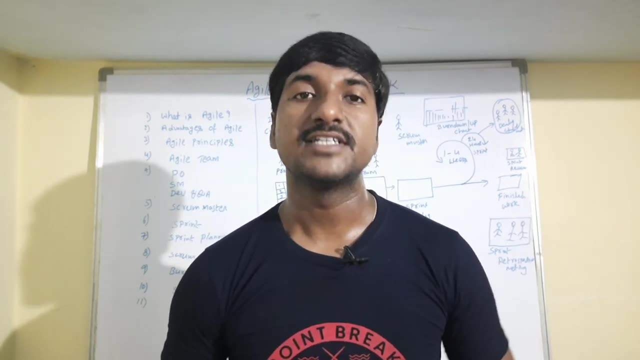 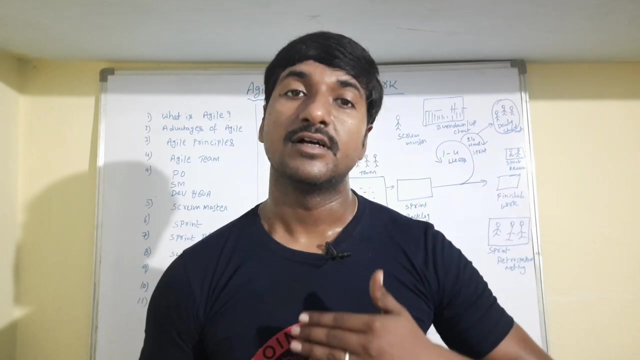 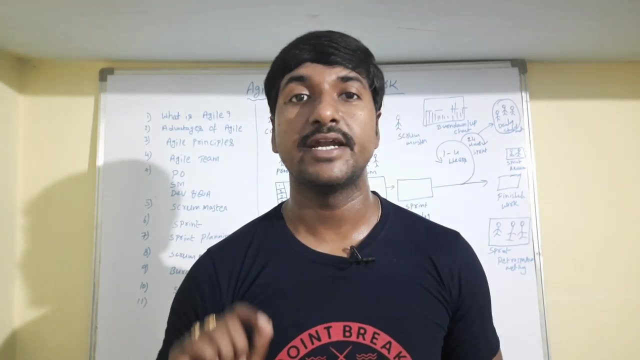 going as for as an principles or not. if anyone facing any issues are, then he will clarify that one and he will facilitating the candidates as well. and one more dev team and qa development team will develop the software and qa team will testing the software. so this is the scrum team: product owner, scrum master and development team, qa team. okay, now we'll. 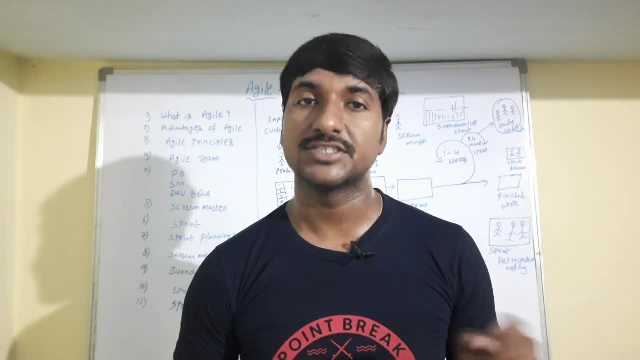 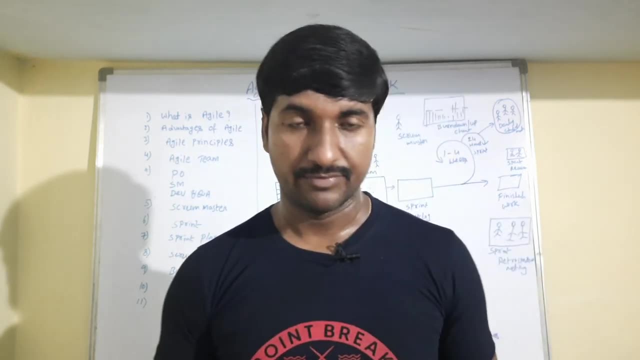 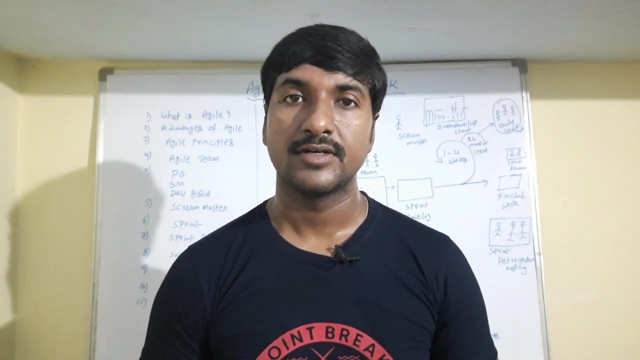 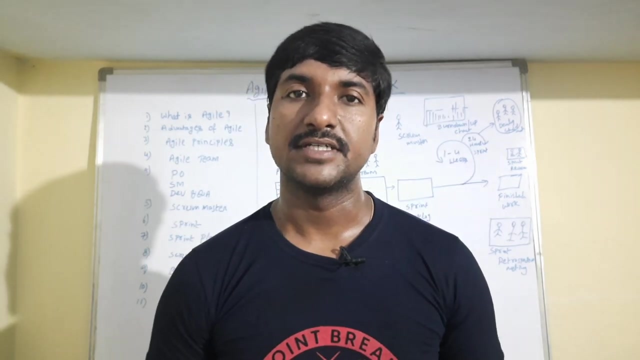 talk about some scrum terminologies. guys like: what is a sprint? sprint planning meeting, sprint review, sprint retrospective meeting, what is a daily stand-up meeting? then, what is a sprint? sprint is nothing, but it is a particular duration of time to complete the user stories. generally, in every it companies, sprint duration is nothing but two to three weeks, guys, you have. 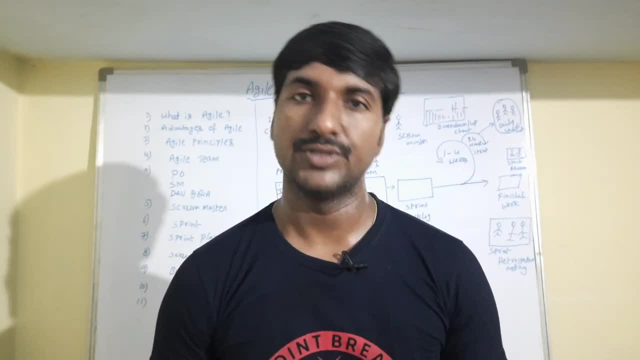 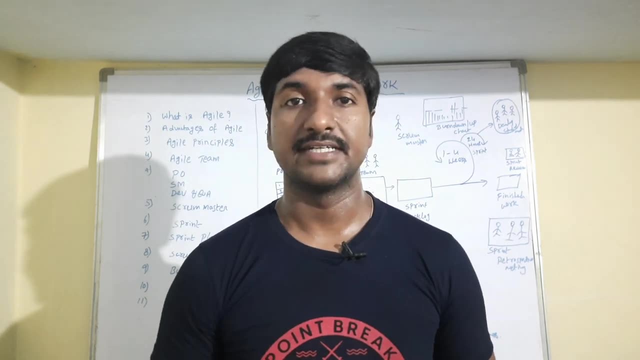 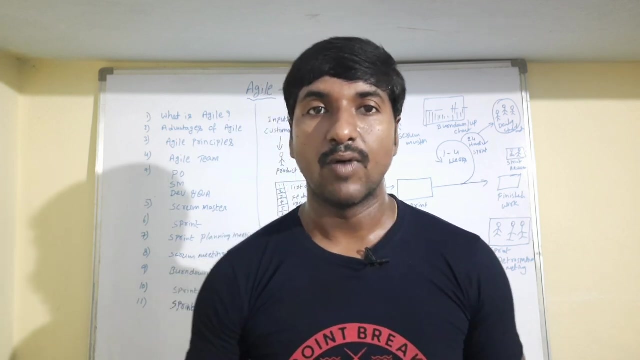 to complete the task. you have to complete the user stories within that time. that is nothing but sprint. now, what is the sprint planning meeting? in the sprint planning meeting? so, as a team- uh, they will discuss in the meeting what. what are the user stories we have to deliver? 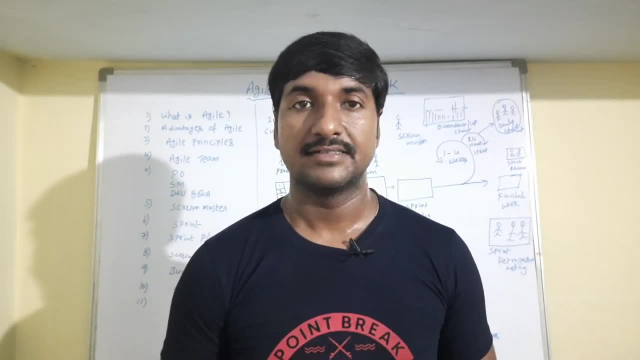 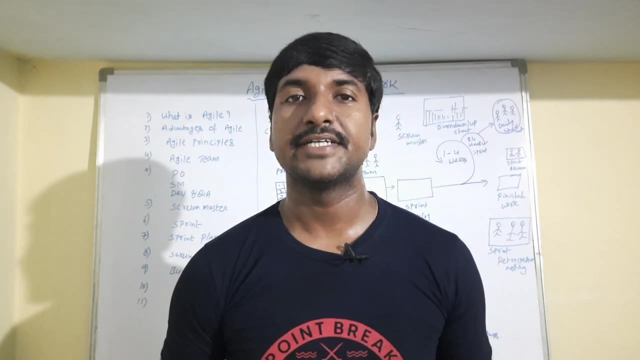 in this particular sprint. and what is the scrum meeting? the scrum meeting is nothing, but it's a daily stand-up meeting. okay, in the daily standard meeting, they will discuss about what you did yesterday, what you are going to do today and what are the other things that you are going to do today. 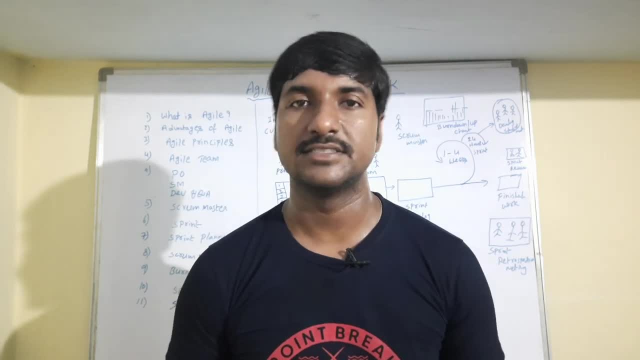 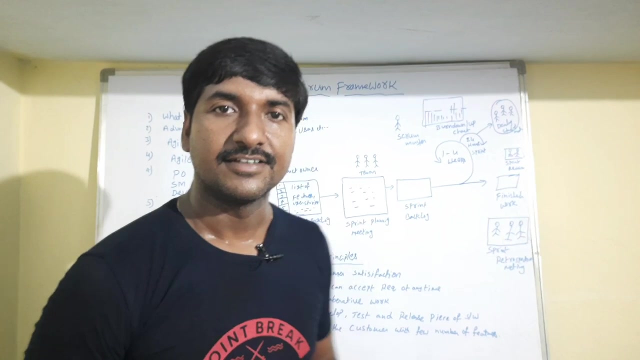 and what are the problems you are facing. so they will discuss these things in the scrum meeting for every day. there are around 10 to 15 minutes of daily stand-up meeting is there. it is conducted by the scrum master. only now let us see the agile project methodology process. okay, first, 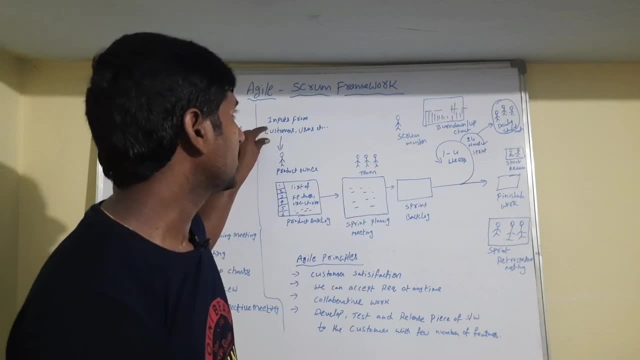 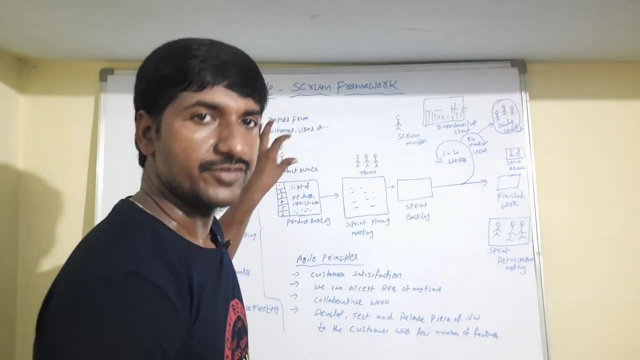 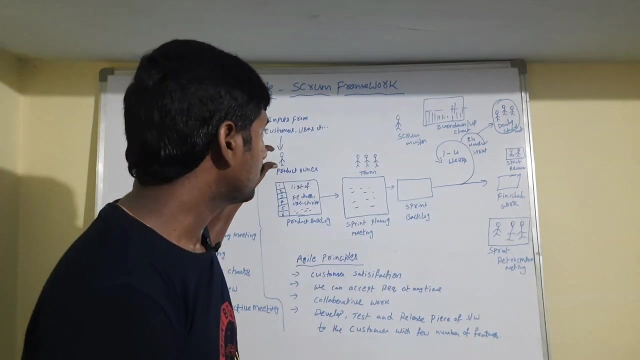 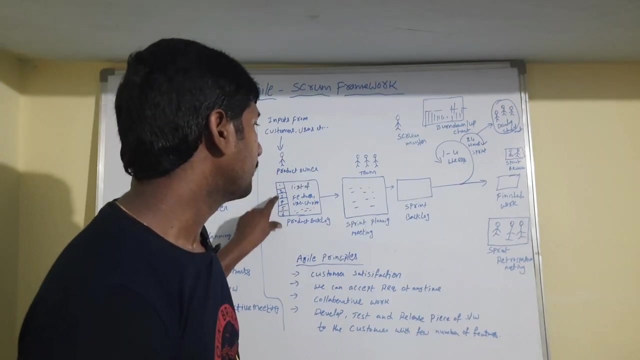 the product owner will take the inputs from the stakeholders or customers or end users. he will collect the user stories or features from the customers or stakeholders or clients. okay, so product owner is responsibility to gather the requirements. okay, and he will prepare one product backlog. product owner: prepare product backlog. 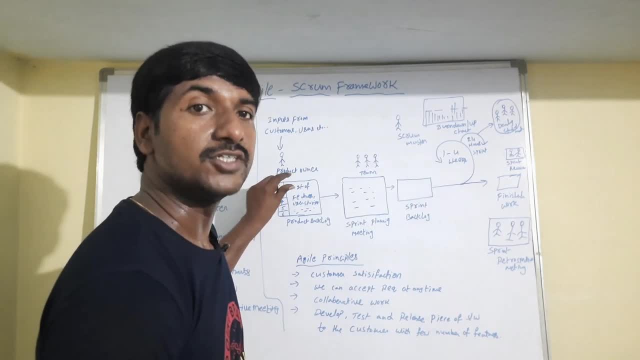 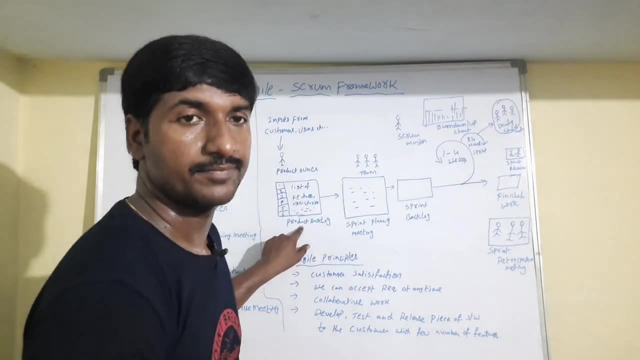 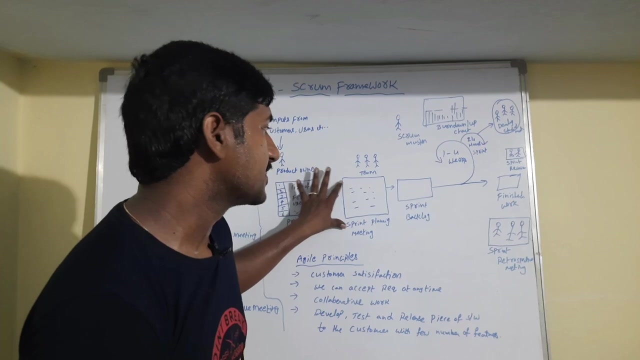 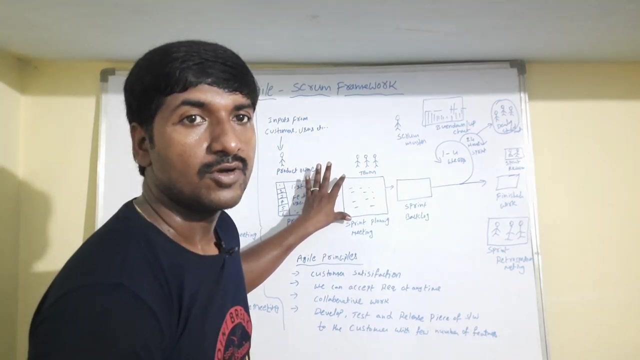 in the product backlog. it contains a list of user stories. it contains a list of user stories. it is. it will be prepared by the product owner only, okay. so after that the team will conduct the sprint planning meeting. in the sprint planning meeting the team will discuss about what are the requirements we have to. 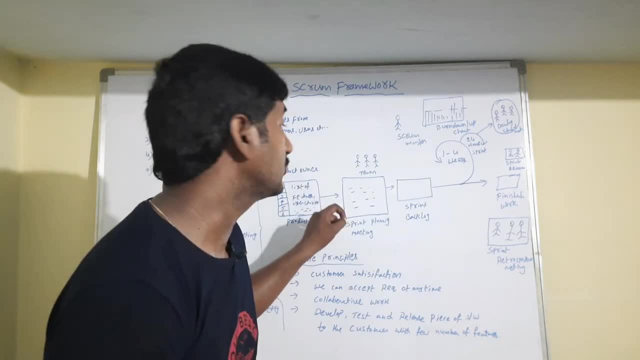 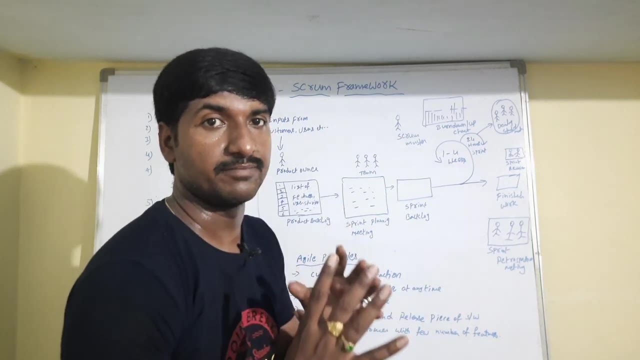 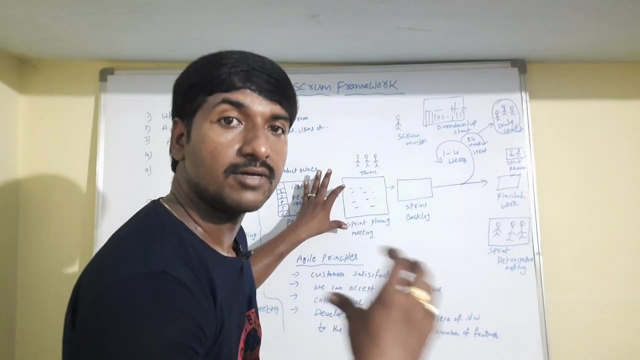 complete. what are the user stories? what are the features we have to complete in this specific sprint? already told you, sprint means the user stories are the user stories that are going to be completed within a certain duration, particular duration to complete the task. okay, so in the sprint planning meeting, what are the? 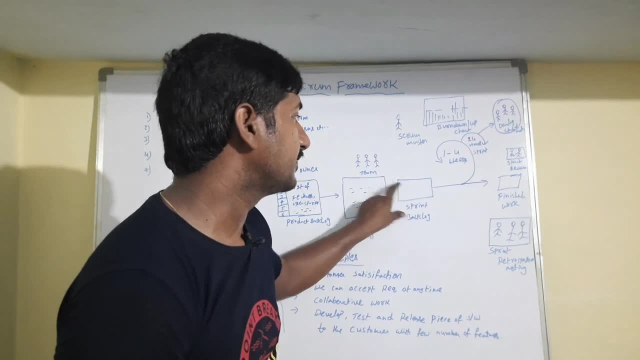 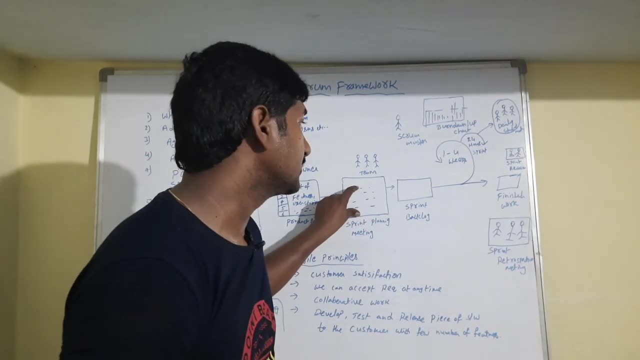 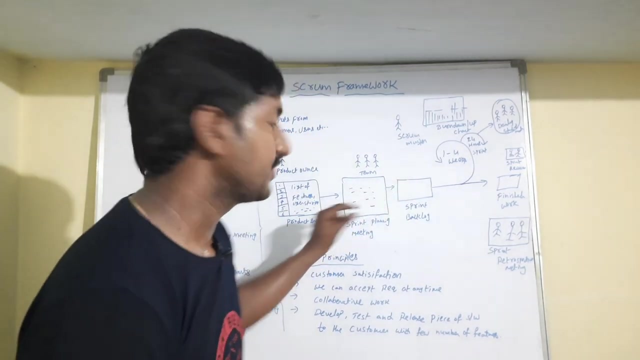 user stories we have to complete. how many number of user stories we have to complete? okay, and then you will. and then sprint backlog. in the sprint backlog it contains: what are the committed user stories? what are the committed user stories are product backlog and sprint backlog. in the product backlog, all the requirements are: 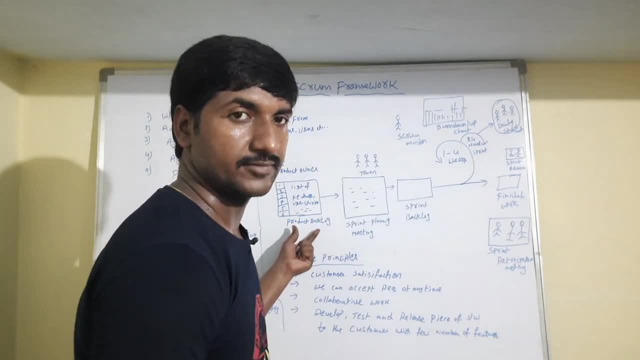 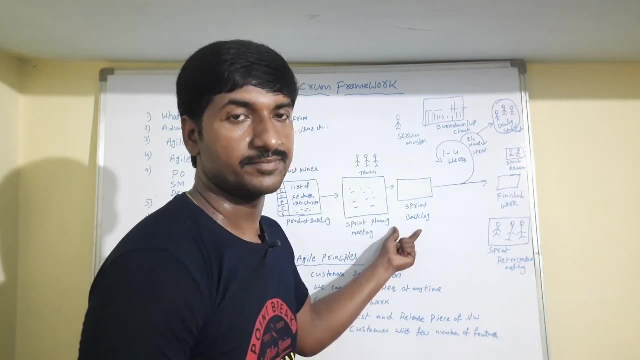 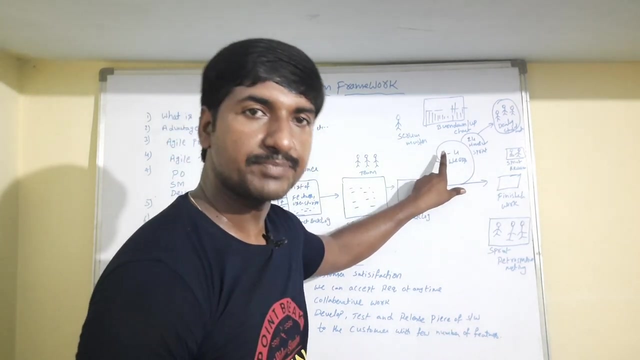 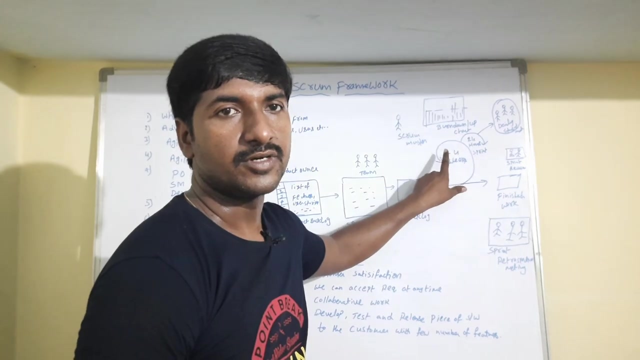 in the product backlog all the user stories available, all the features are available. but in the sprint backlog only the committed user stories or features are available. okay, and then a sprint will start. so the sprint will start. so usually the sprint duration is one to four weeks, okay, maximum companies will follow. two to three weeks, guys, okay, and for every 24 hours. 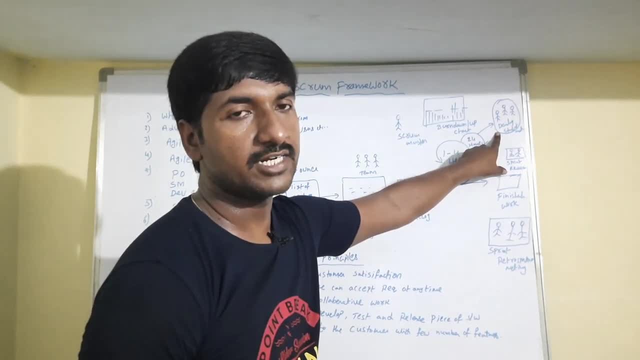 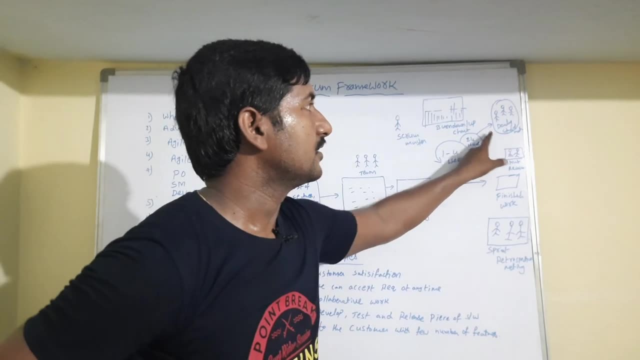 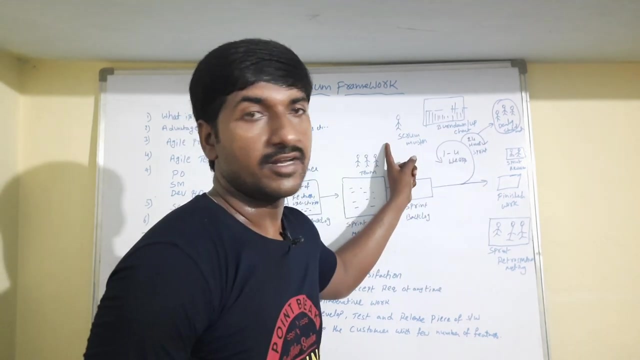 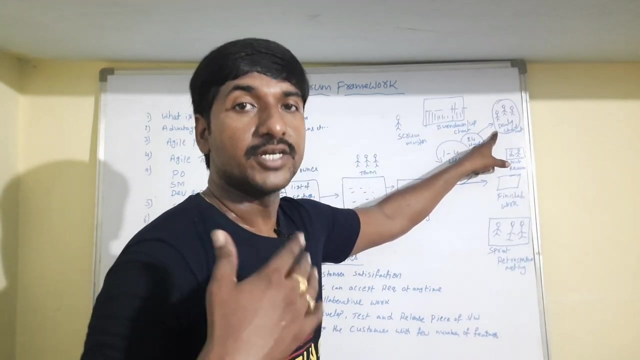 one daily stand-up meeting is there. who will conduct this daily stand-up meeting means scrum master. okay, scrum master will discuss about. so scrum master will ask for each individual candidate. scrum master will ask for each individual person about what you are doing, did yesterday, what you are doing today and what is the issues are there? so he. 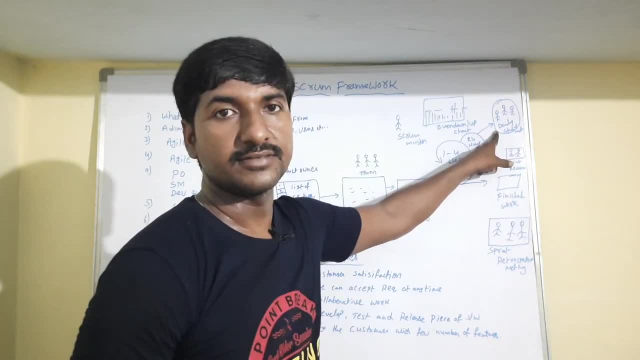 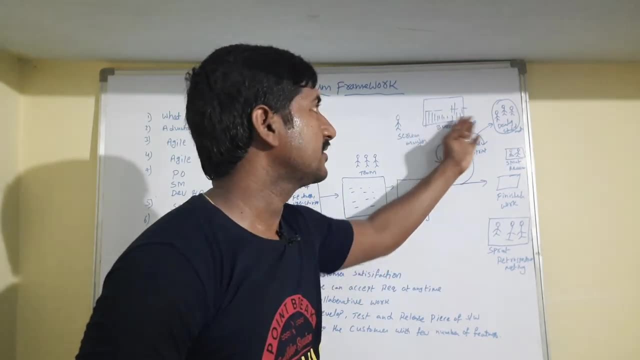 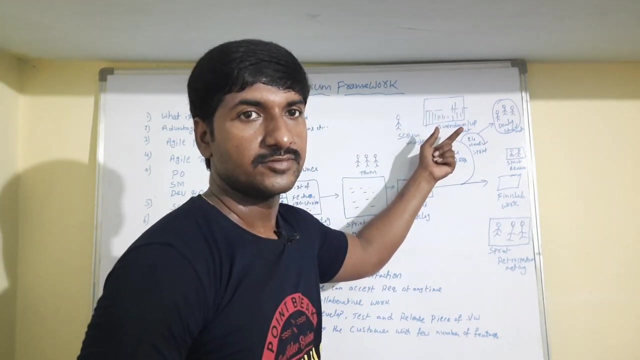 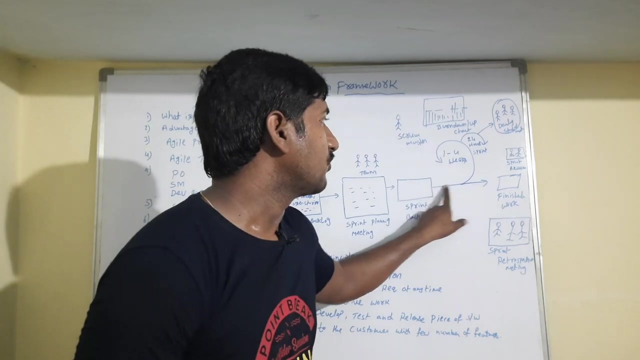 will discuss each and everything in 15 minutes in daily stand-up meeting. and also scrum master will prepare one burn down and up chart. so, based on their feedback, he will prepare one graph in the form of graph. so, based on this burn down and burn up chart, we can analyze the performance of the product. so 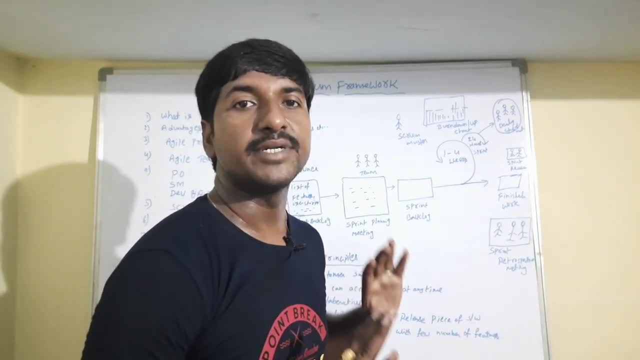 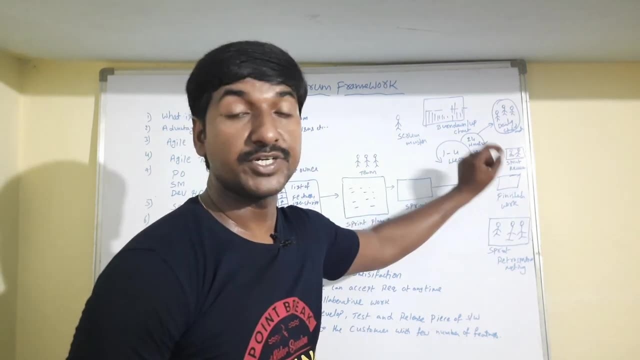 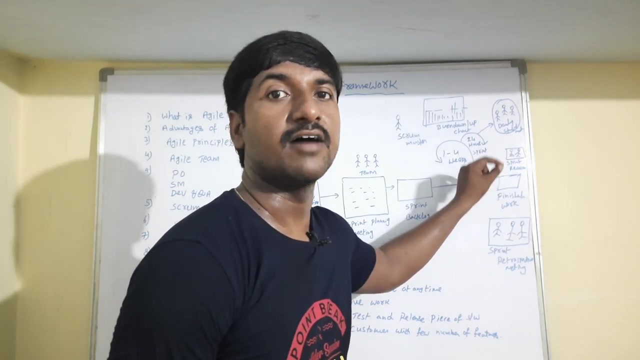 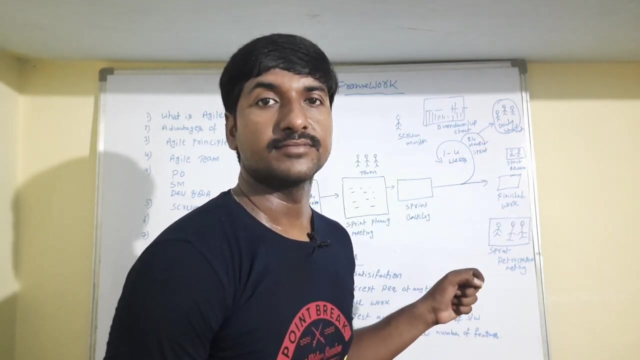 once you finish the work, that means you completed your first sprint. so then you will conduct the one sprint review meeting. in the sprint review meeting you have to show demo to the product owner, whether it is working as per our requirement or not. here product owner may accept or reject your sprint. 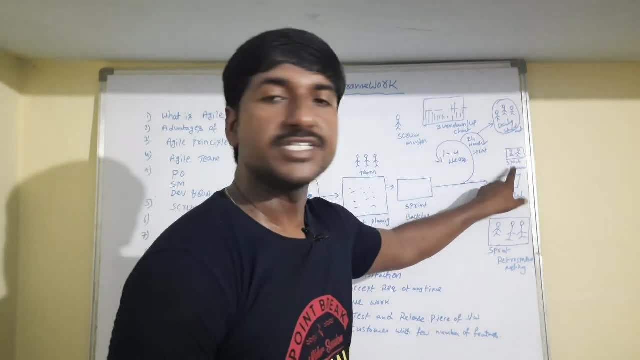 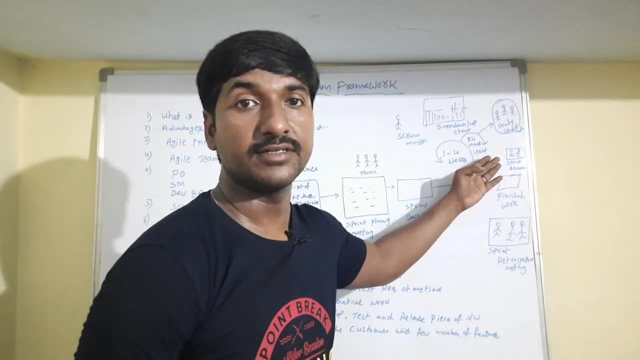 okay, so in the sprint review, each and everything will check it out. okay, so in the sprint review, each and everything will check it out. okay, so in the sprint review, each and everything will check it out. okay, after that, after sprint review, meeting and one more meeting is there. 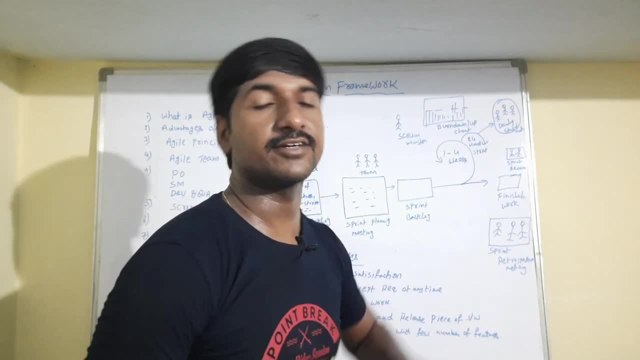 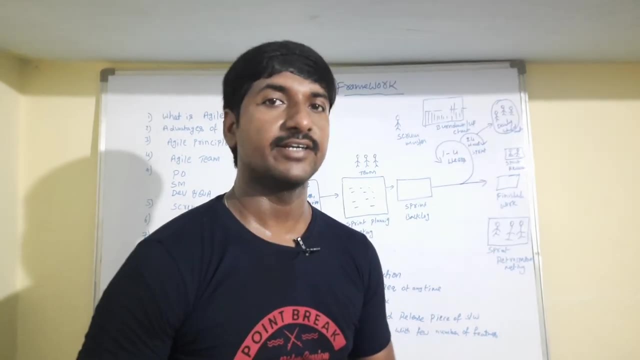 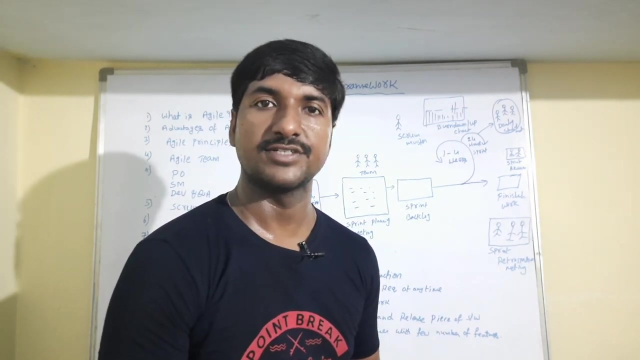 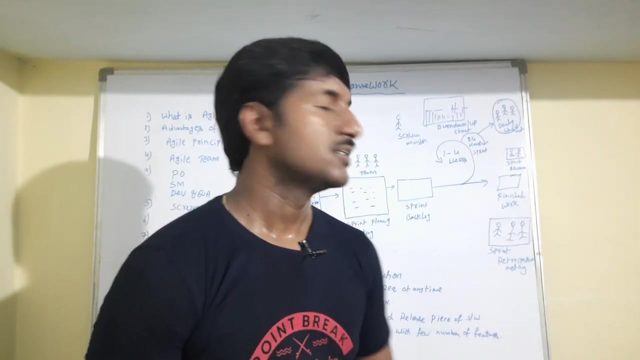 guys. sprint retrospective meeting. in the sprint retrospective meeting the team will discuss about what went well, what went well and what went wrong, how the performance of the last sprint. is there any issues we faced? what type of issues we faced, where we struggled, how you overcome those issues. so then will discuss on these things about a last sprint, okay, so 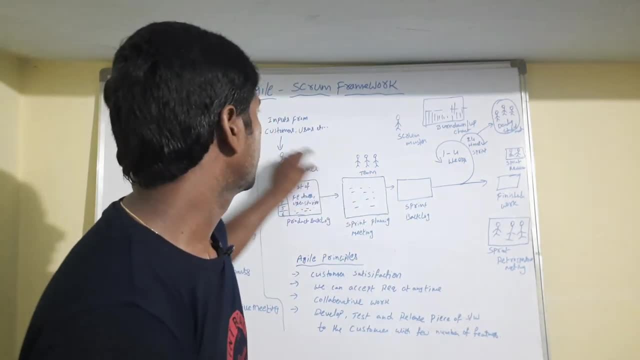 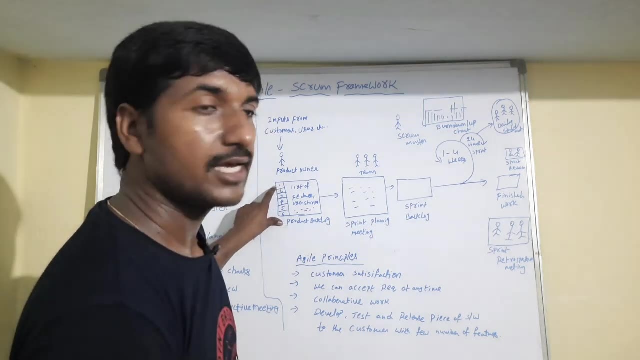 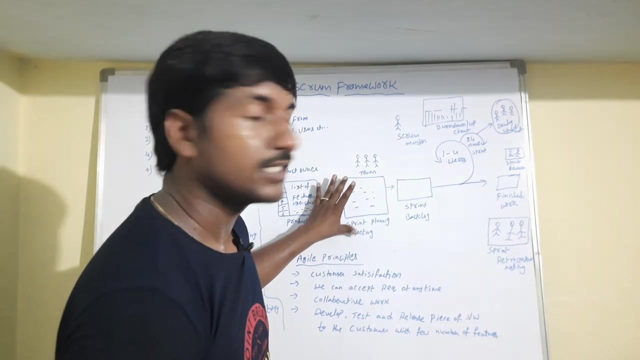 this is overall the action project process case. okay, product owner responsibility to take the input and he will prepare on product backlog. in the product backlog it contains a list of requirements and and then team will conduct one sprint planning meeting. in the sprint planning meeting they will choose: they will choose the requirement for a sprint planning meeting and he will choose the requirements menu. 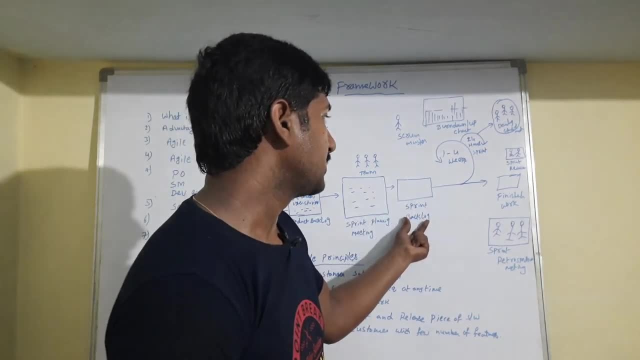 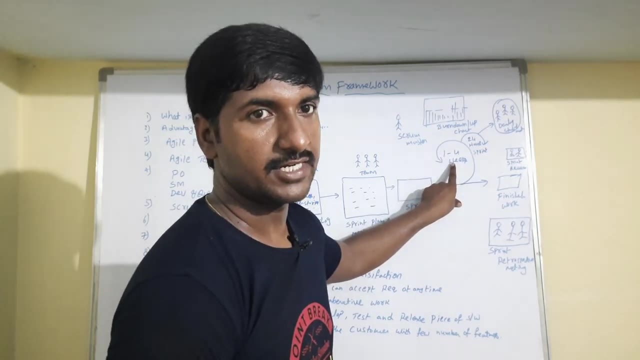 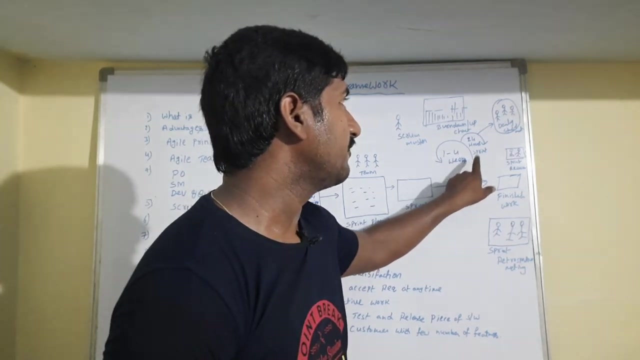 from the list of features and then in the sprint backlog the committed requirements are available and then you will prepare one sprinter. one to four weeks, generally two to generally two to three weeks are there for every sprinter in IT companies into, okay, for every 24 hours of one daily stand-up meeting is. 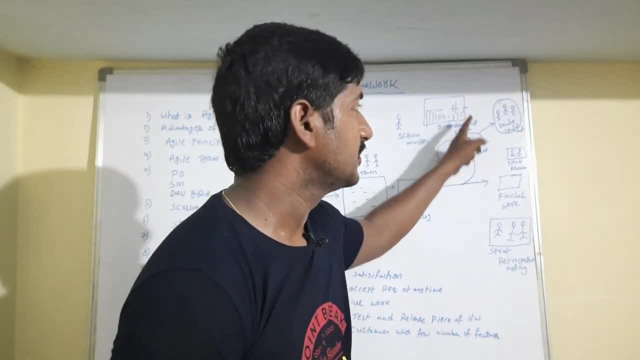 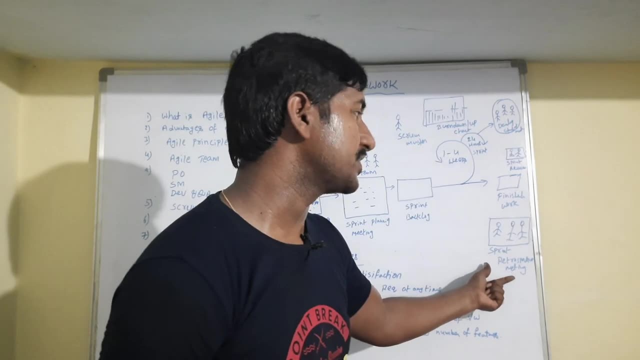 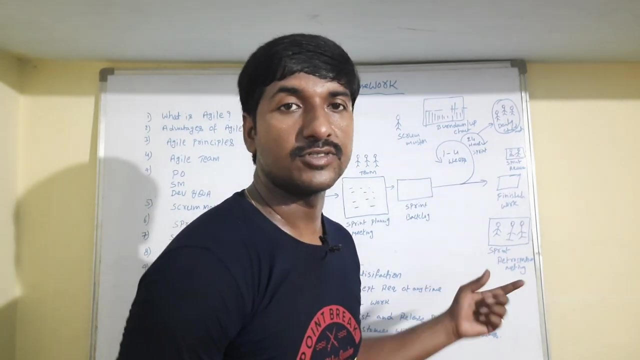 there. this is conducted by the scrum master only, okay, so after finishing a work. so they will take the one sprint review meeting and one more meeting is the sprint retrospective meeting in the in this rate in this meeting. in this meeting, the team will discuss about what went well, what went well and what went. 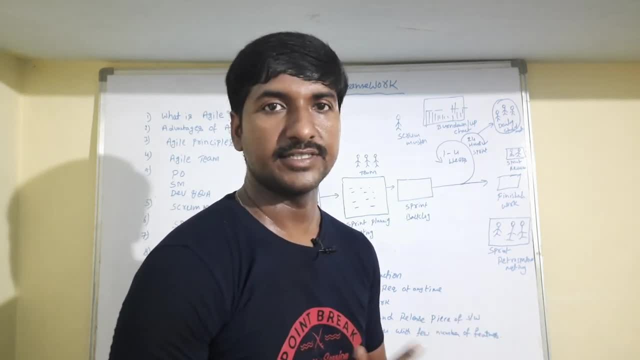 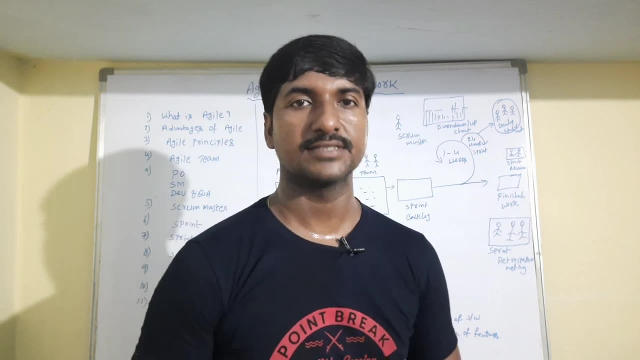 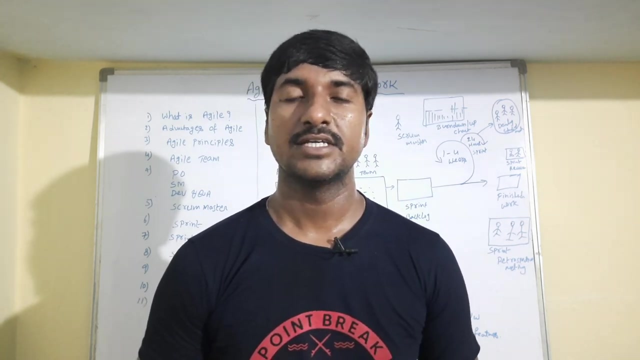 wrong? okay. is there any issues? are there in the last print? how to overcome those issues? these are the discuss in the sprint retrospective meeting, guys. so that's all about guys, about the complete sprint review agile process, guys. okay. so if you have any doubts, please comment in the comment. 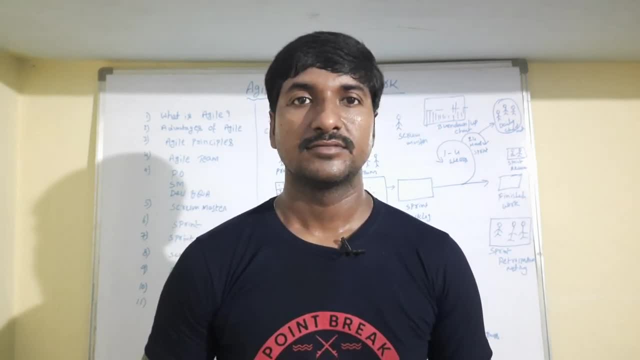 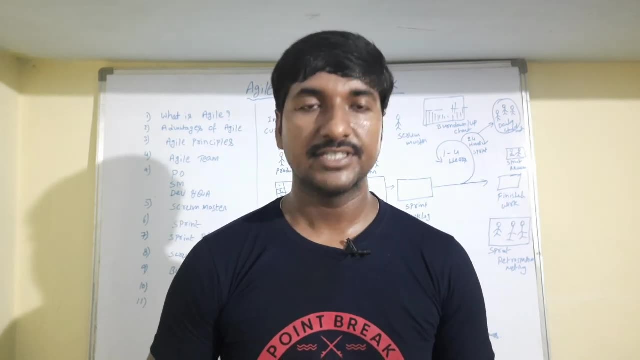 box I will reply to your queries. so if you feel this video is very helpful, please share to your friends also, guys, so we'll meet in the next video. thank you very much.